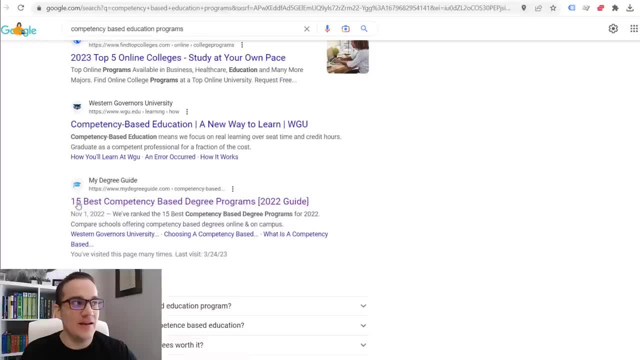 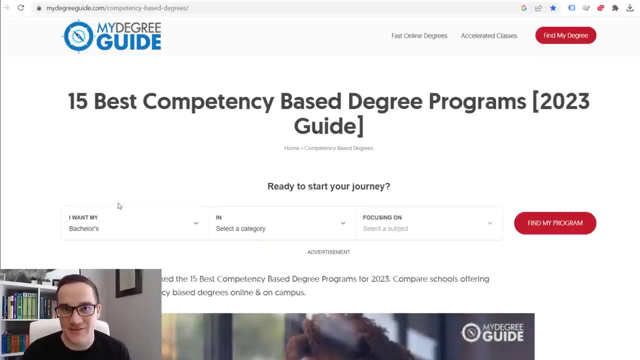 And then you're going to see a whole bunch of advertisements. Then there's this website called My Degree Guide. Every year they post a list of like 15 of the best competency-based education programs. We're just going to go there and you're going to start with 15, okay, There are more than. 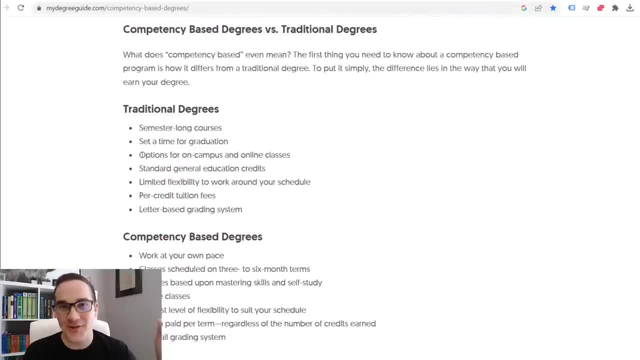 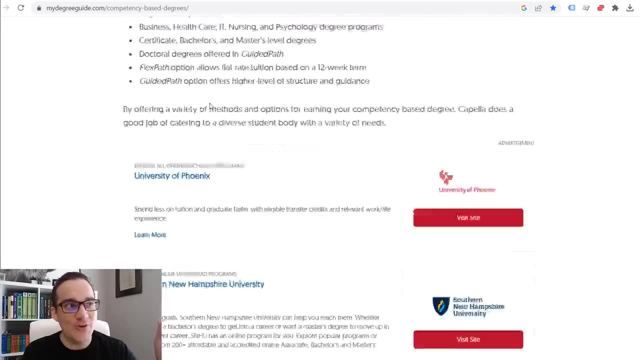 this, but this is a really good place to start Now. if you start the article you're going to scroll down. there's ads everywhere, Like seriously, there are ads everywhere. But if you keep scrolling, like near the bottom of the article, you're going to see this section, that 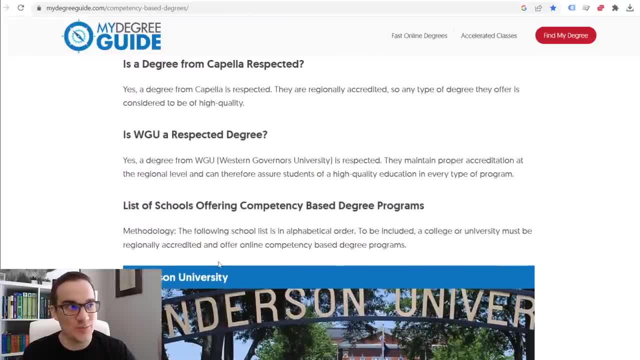 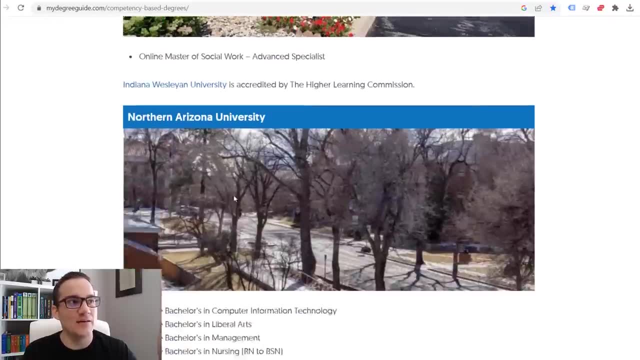 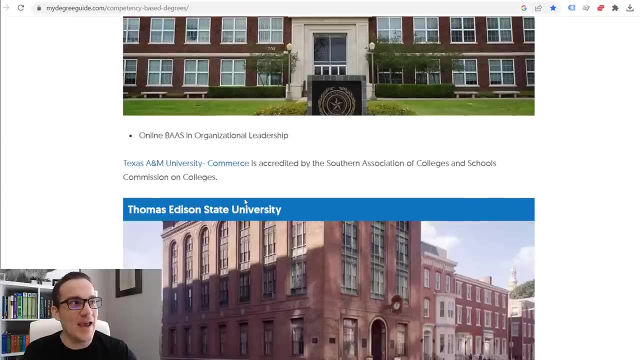 says list of schools offering competency, competency-based education programs, and boom, there's a big list: anderson university, capella, indiana, wesleyan, northern arizona, purdue university, global rasmussen college, southern new hampshire university, texas a&m, thomas edison state. 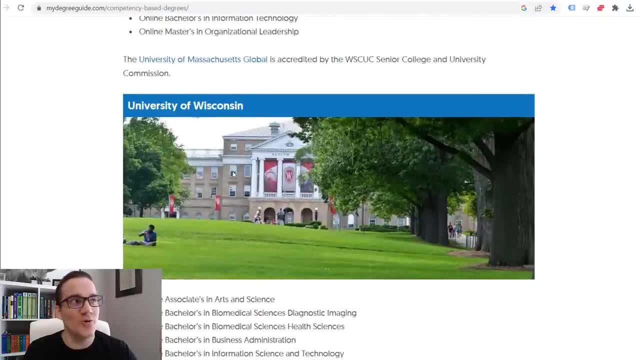 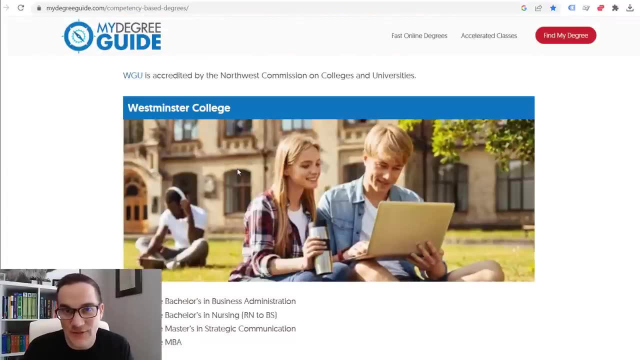 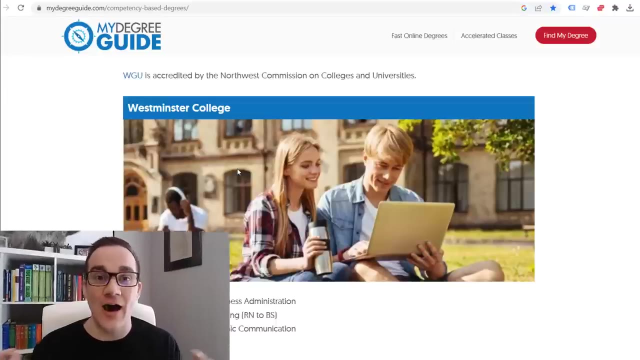 university of louisville, university of massachusetts, global university of wisconsin, walden western governor's university, westminster college- there's like that's 15 competency-based education programs right here and this is a really, really good place to start now. this is debatable in the online world if you're looking how to get a college degree faster. 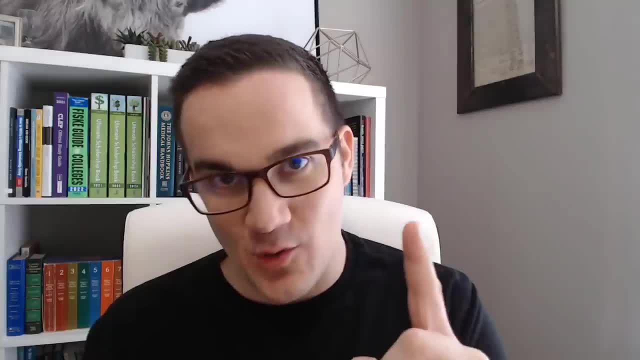 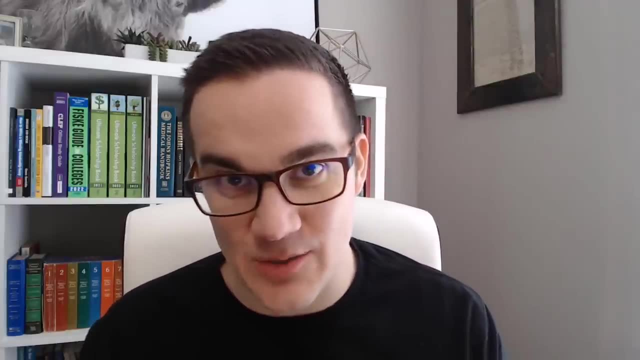 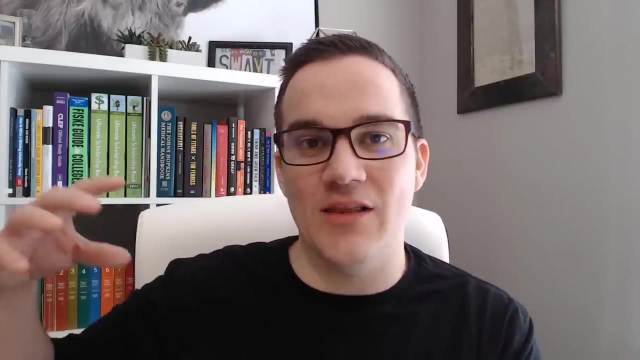 there are two ways to do this way. number one: the strategy that i highly prefer is to do this way. number one: the strategy that i highly prefer is to do this way. number one is to enroll in a really rock solid, competency-based education program and test out of all your classes through the university. strategy number two is to go online. 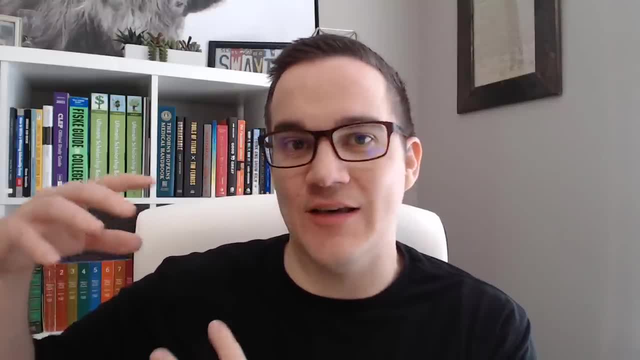 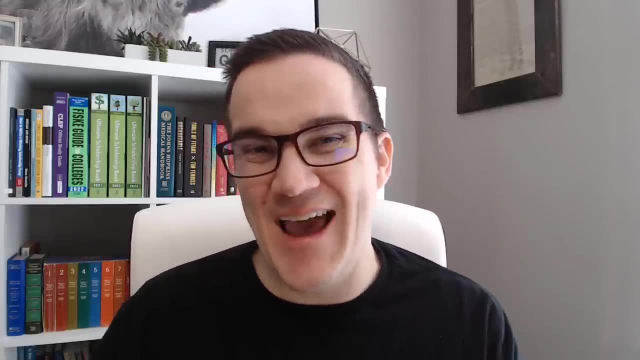 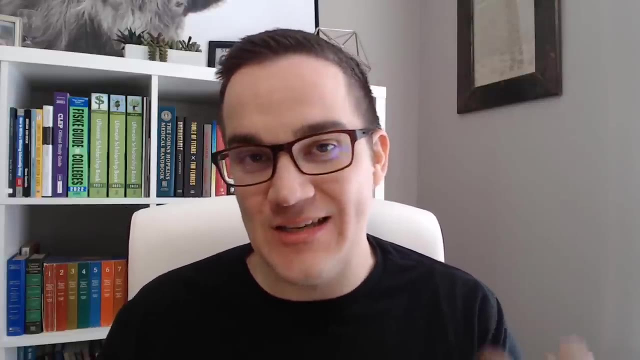 and buy a bunch of third-party college level exams, take a bunch of exams through third-party resources and then transfer them over to universities that have really, really lax standards for what they'll accept for transfer credits. and there are universities that will accept like three years worth of college credit from third-party resources, and you've maybe heard 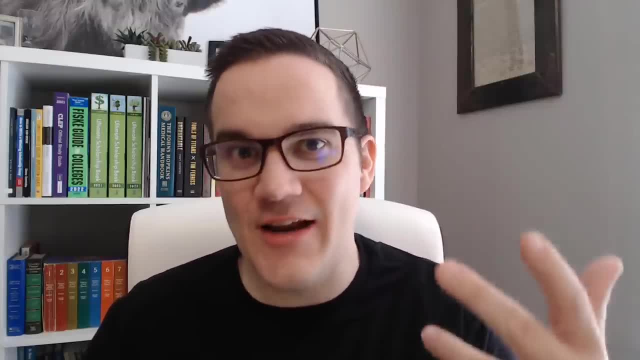 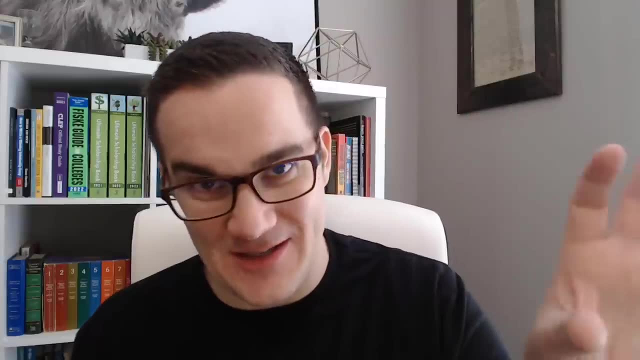 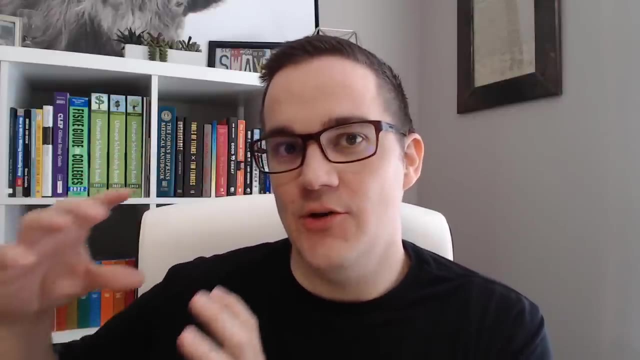 of this. it's like cLEP exams, sofiaorg, studycom. there are a bunch of different resources where you can do this. i prefer competency-based education programs because it's faster. okay if you go and hack like three years worth of school through these third-party resources. and then transfer credits over to a university, you still have to do a year worth of school school the normal way. So instead of being able to graduate in like six to 12 months, you're looking at closer to like two years. Okay, And most schools have that requirement. 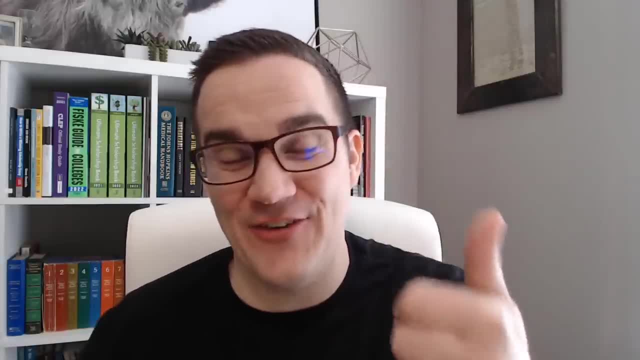 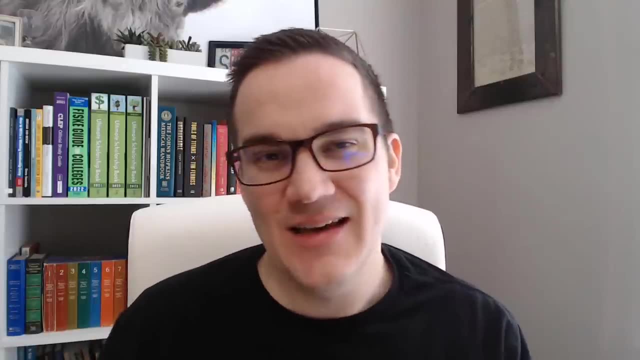 will let you accelerate most of your degree, but you have to finish at least a year of of your education through our program. So when you're doing the transfer strategy, it's it's not as fast, Okay, And when you're doing it through university. 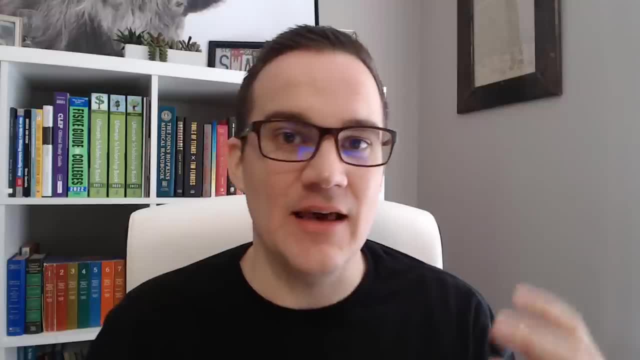 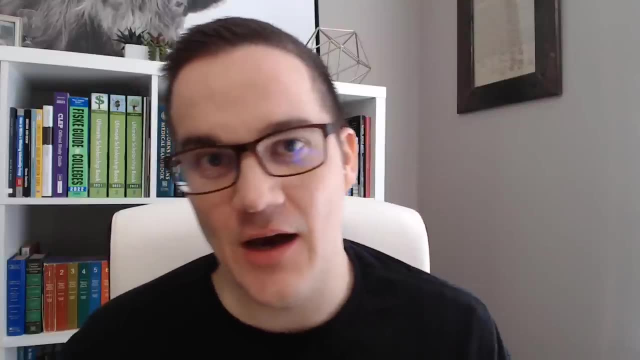 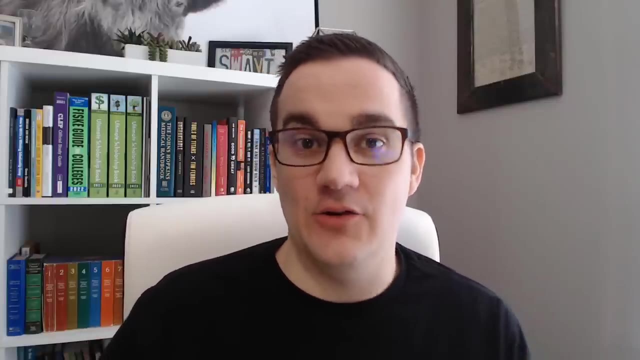 there are some really rock solid schools that allow you to do this, So you usually end up with a higher quality degree anyway. Okay, So that's number one is you find a competency-based education program. Number two: you find a program that you like, once you've found a competency-based 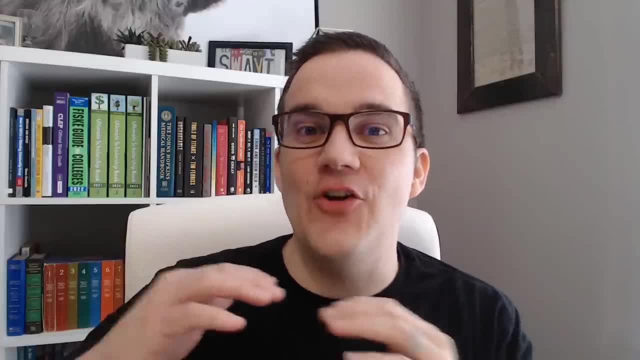 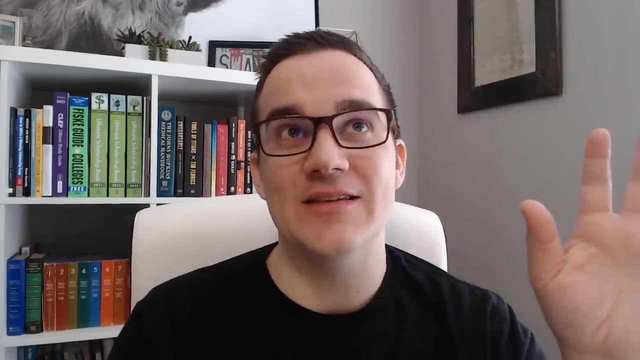 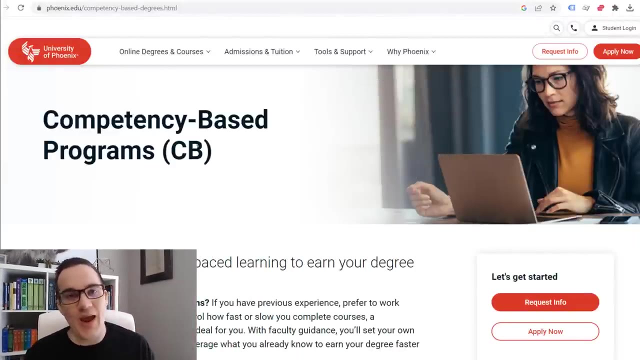 education program. you want to make sure that they have no restraints on how fast you can graduate, zero time restraints. Okay, Now I'm going to give you an example. I'm going to show you a bad example. Okay, University of Phoenix. Okay, They claim to have 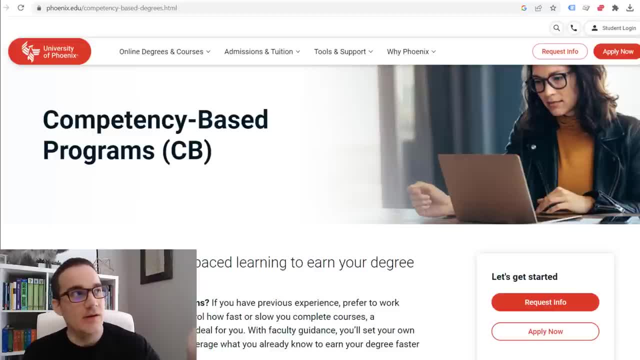 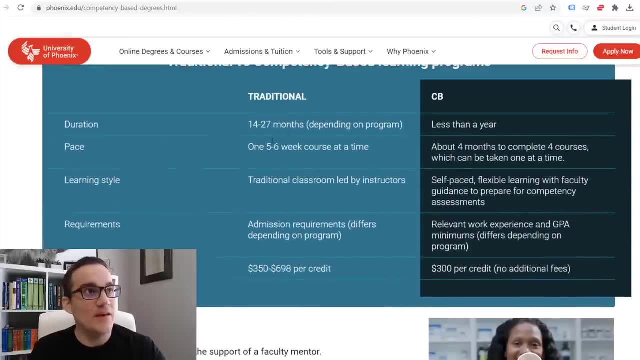 competency-based education programs. This is their page where they talk about their competency-based education programs. If you scroll down, they're going to give you a little more detail, And if you look at this section that says pace. their traditional programs are one, five to six week course at a time. Okay, Or their competency-based programs. 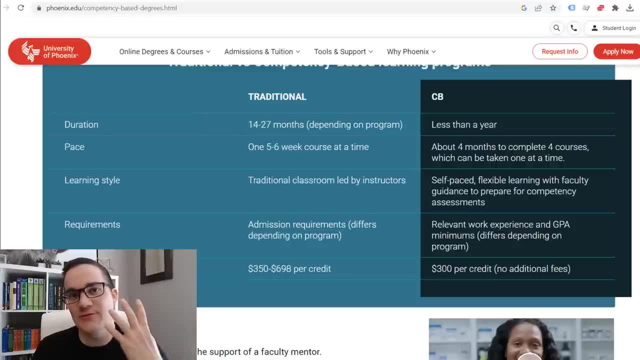 are about four months to complete four courses. Okay, So it's your. your time restraint is one class per month, essentially Okay, Well, just being able to go at your own pace or finish classes at your own pace. it's not helpful if they cap how many classes you can complete. 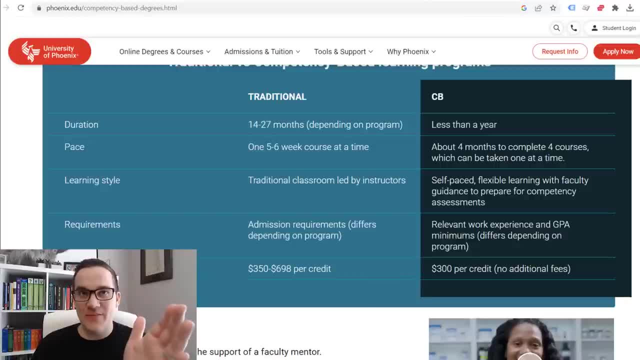 per semester. Okay, Four semester or four. four months to complete four courses. That's traditional pace. Like most semesters are four months long and you usually take four or five classes. Okay, That's how college normally works. So instead of 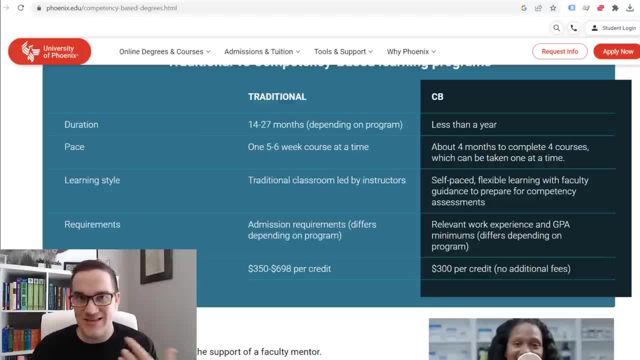 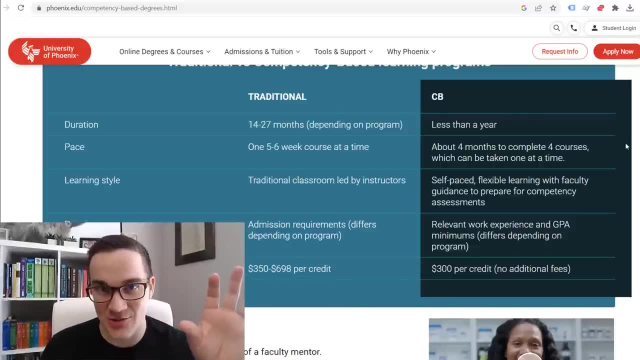 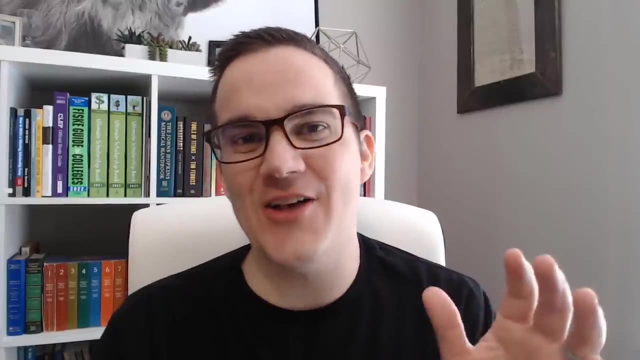 like going through four classes at the same time. you're going through one class at a time, but it's taking you just as long. Okay, This is a perfect example of what not to choose. Now. I have had some feedback Like I did a video on this in the past and someone said: that's not. 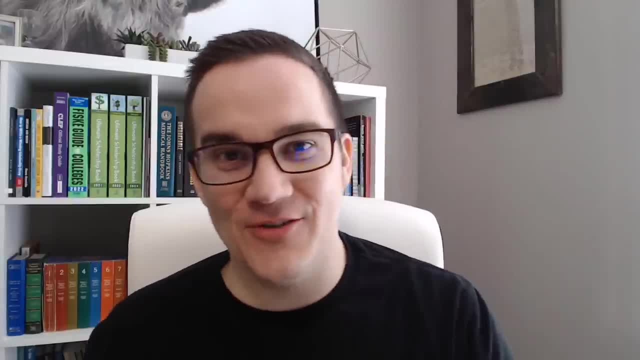 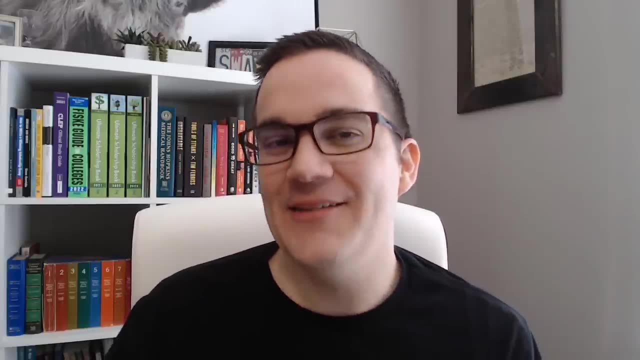 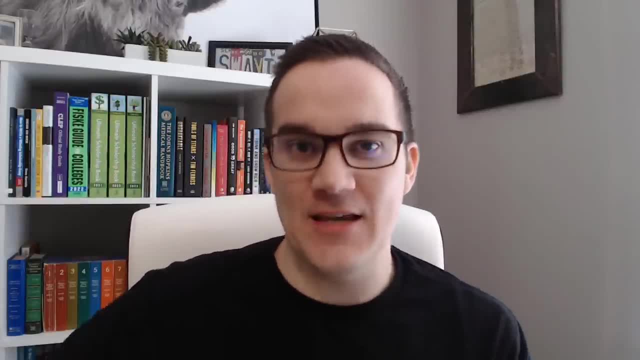 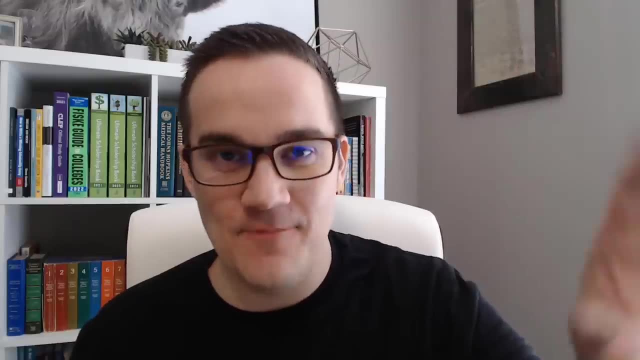 classes in four months instead of four classes in four months. Guess what You're going to graduate like three months faster, but it's still going to take you more than four years. Don't, don't, bite, Okay. What you're looking for are universities that literally like 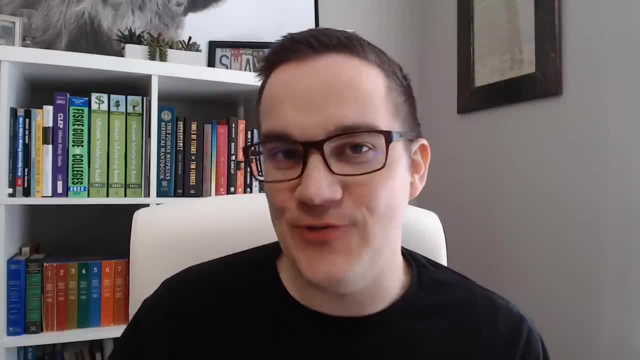 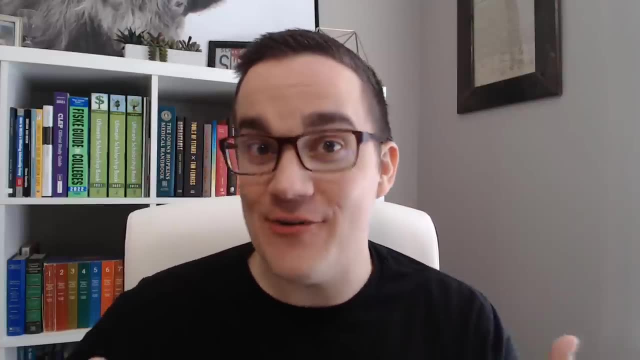 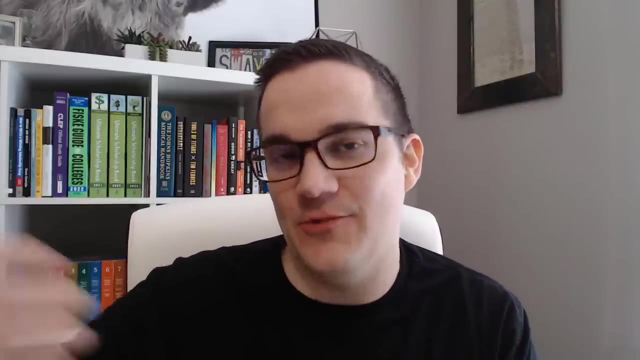 you're going to enroll in a semester and they will allow you to finish unlimited classes per semester. If you finish one class in a day, they will give you credit for that. one class in a day. If you do a class a week for an entire year, they will let you graduate. You'll graduate before that. 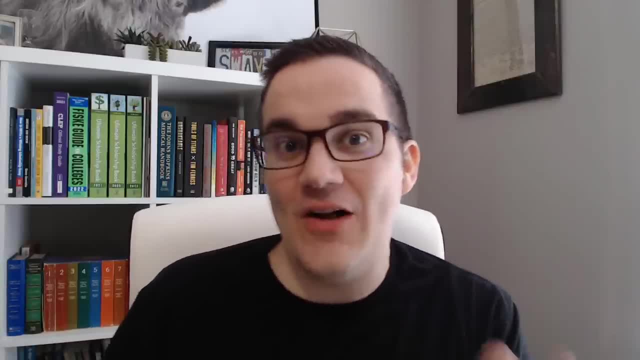 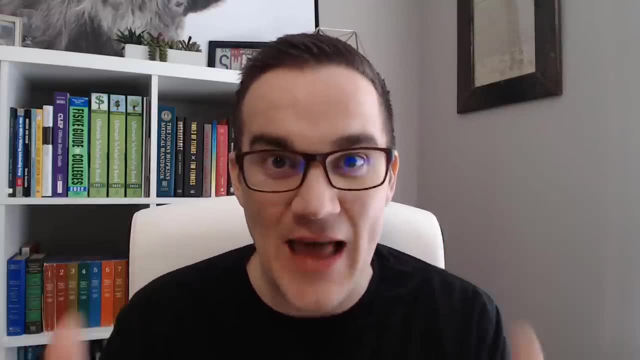 because a bachelor's degree is normally 40 classes. If you did a class a week, which that's what I did, actually- I graduated in nine months and the school had no issue with that. They allowed me to do that. So if you do a class a week, you're going to enroll in a semester and they will allow. 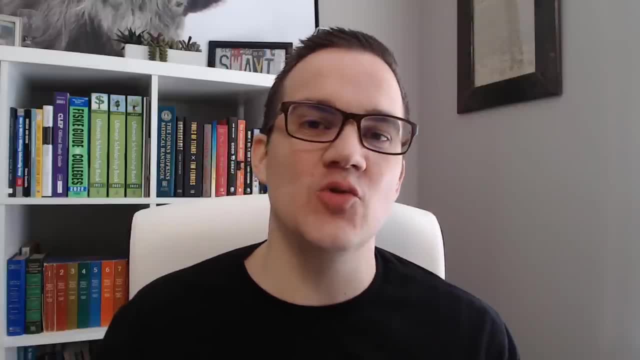 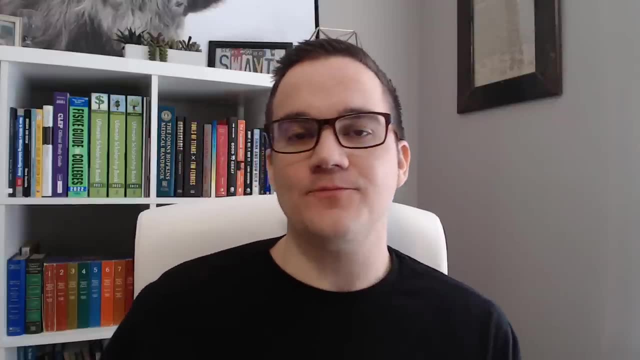 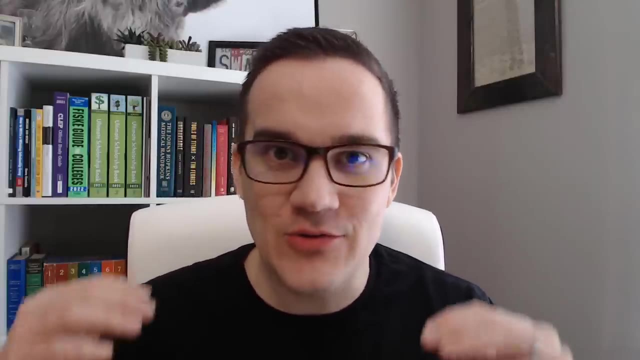 you to do that. So that's step two is make sure the school doesn't have any time restraints on how quickly you can complete classes. Okay, Now number three, and this is really important, because not all schools allow you to do this, but there are really really good schools that do. 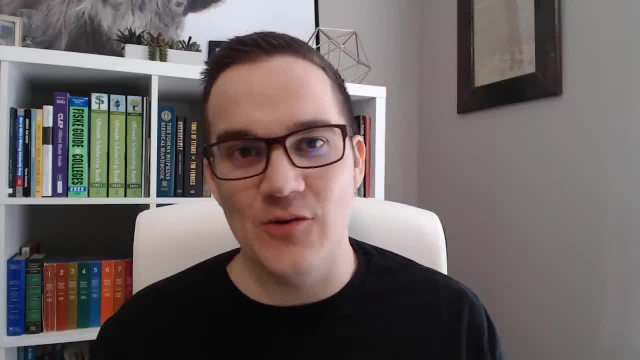 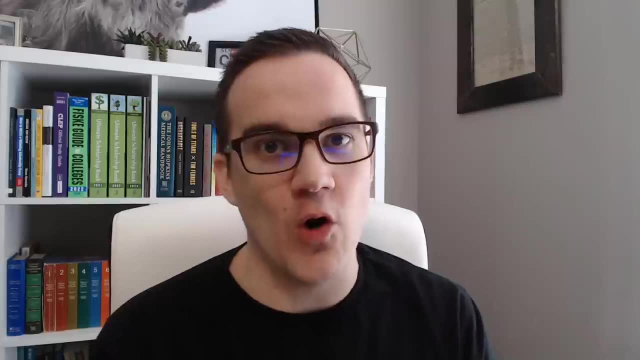 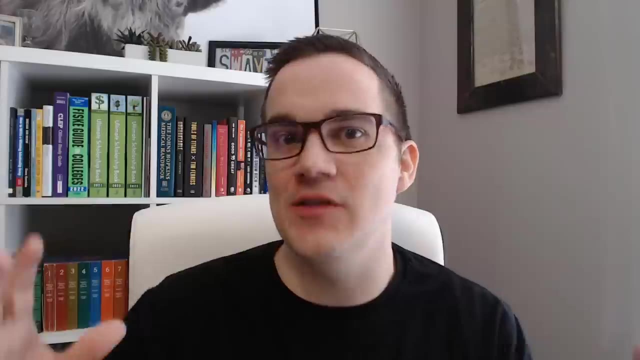 Okay, So the the third tip I want to give you is to just forget. forget about prestige. Okay, A lot of times we like grow up in a certain area. I grew up in Utah and my whole life I wanted to go to the university of Utah. It's like the best school in the state. 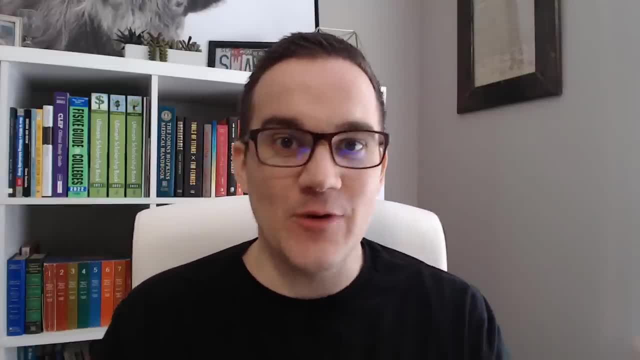 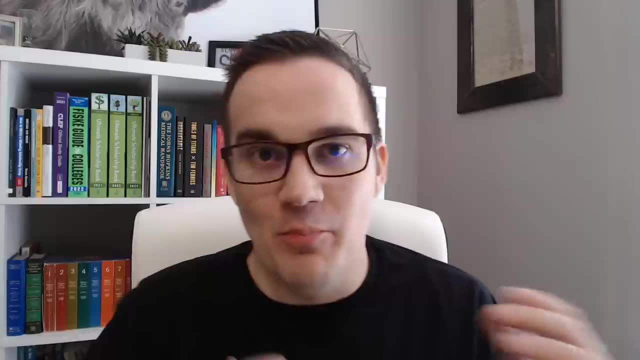 right Or one of the best schools in the state. Now, that's what I wanted. University of Utah does not allow you to get a bachelor's degree in six to 12 months, but there are schools that are equivalent in quality of education that will. 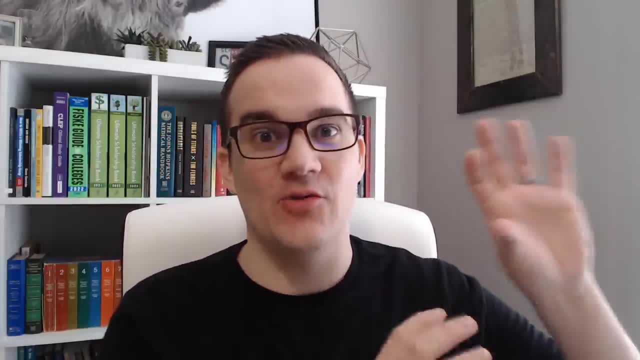 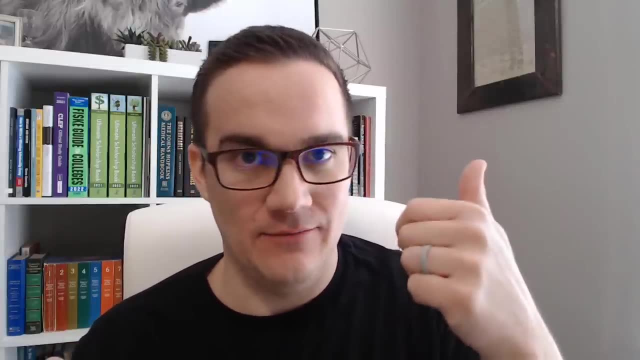 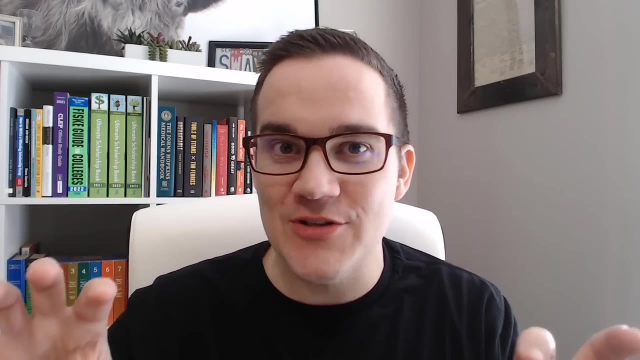 So stop focusing on like I want a degree from this particular school. If you find two schools, one allows you to graduate in six months and one's going to take you five years, but both of those schools open the exact same doors for your career. 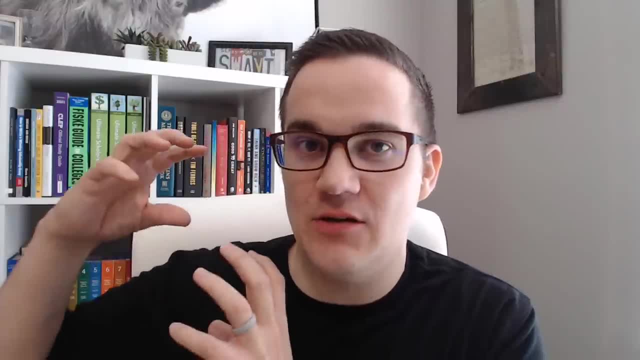 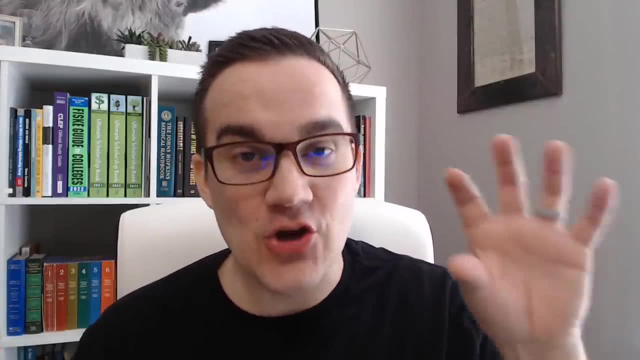 Choose the one that lets you go faster instead of being stuck. And I guess, instead of grasping on to the name of the school, you're going to get a bachelor's degree in six months, So that's that you can have a good, high quality degree like a legit, rock solid, good name degree that. 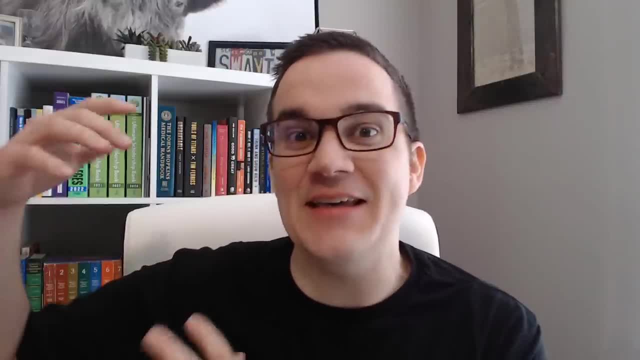 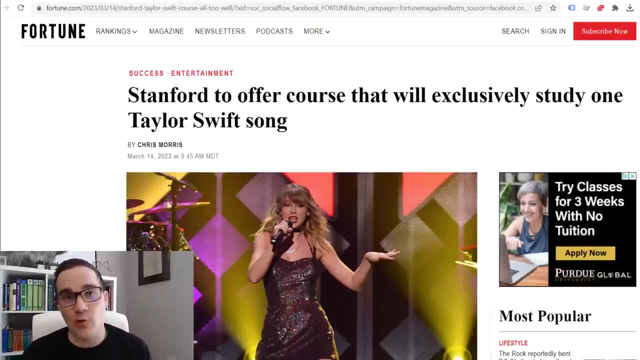 opens the same doors, but it's not the exact school that you're going for Now. I want to give you an example Now. this is an article from fortunecom. Okay, Huge, huge news outlet. This is absolutely crazy. Okay, Stanford university. 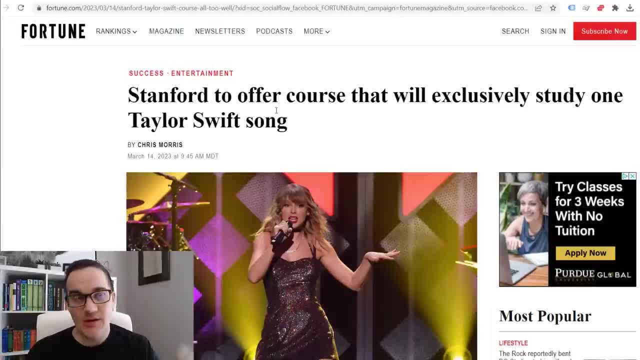 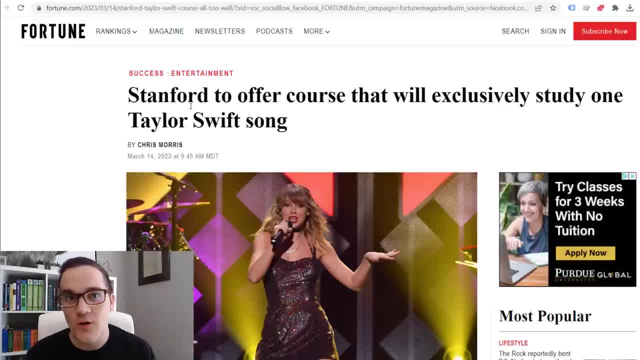 and if you research more on this, I can leave this article down below. but literally, Taylor Swift has a song and there is a four month college class dedicated to dissecting the lyrics of the song and studying what everything means in the song. Okay, So if you're like going, 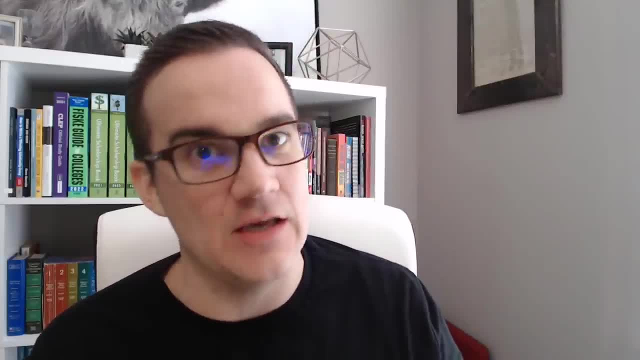 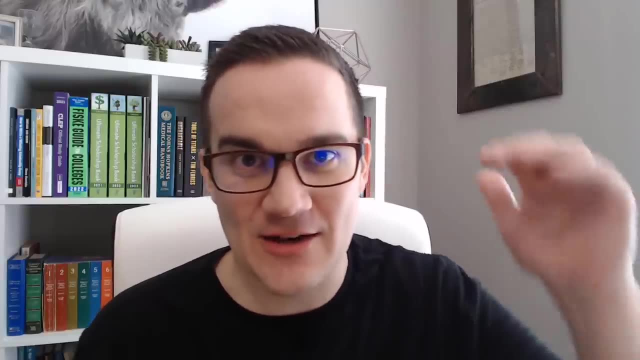 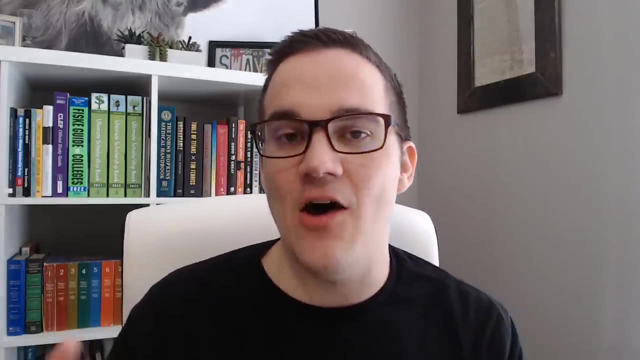 for prestige if you're wanting to go to, like this huge Ivy league big name school, these schools. the quality of education is not necessarily better at these schools, It's just the prestige and the value of the name of the school. Okay Now, having said that, 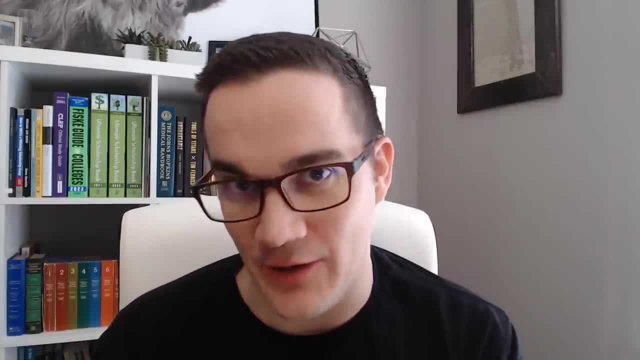 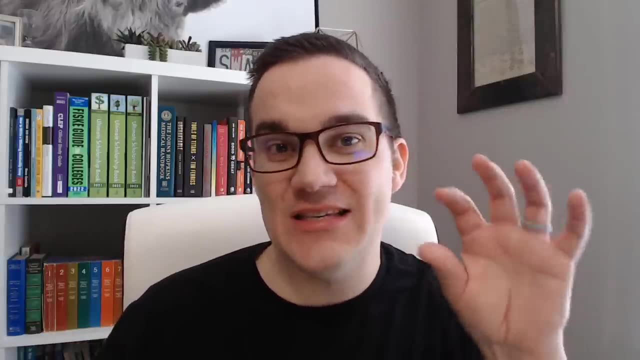 there is a strategy: If you need an Ivy league degree, like if you need to graduate from Harvard to get the job that you're trying to get, you can still hack an undergrad and then transfer over. Okay, Now here's a good example. 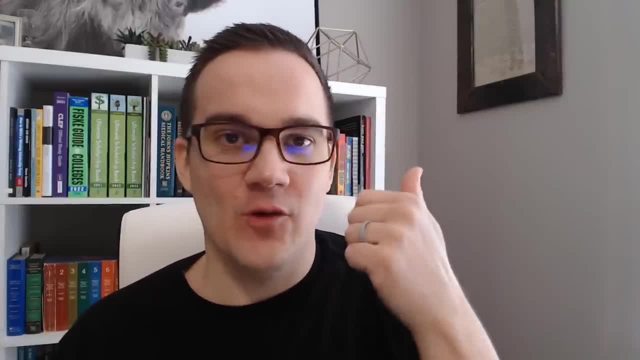 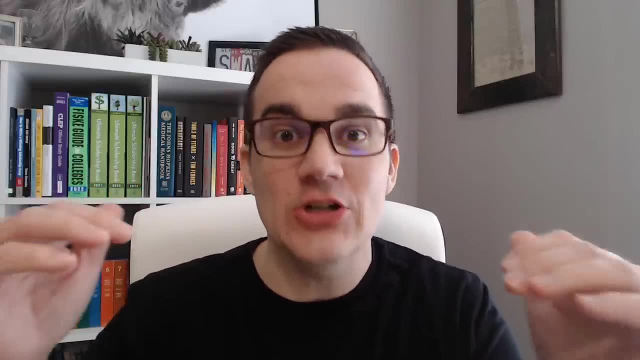 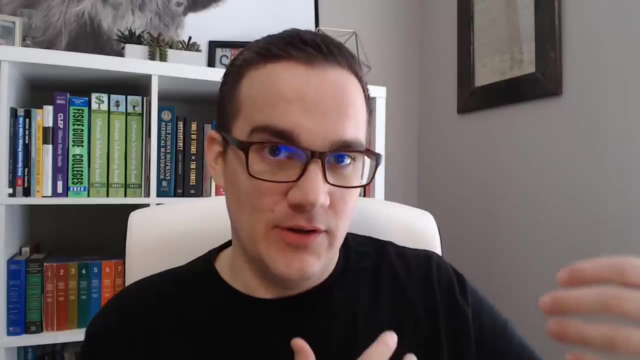 When I'm looking for prestige, I'm looking for what schools have really really good track records for job placement, Like, do their students get really good jobs? And number two, do really really prestigious schools value the these degrees as equivalent to anywhere else? Okay, Let me explain what I mean here. 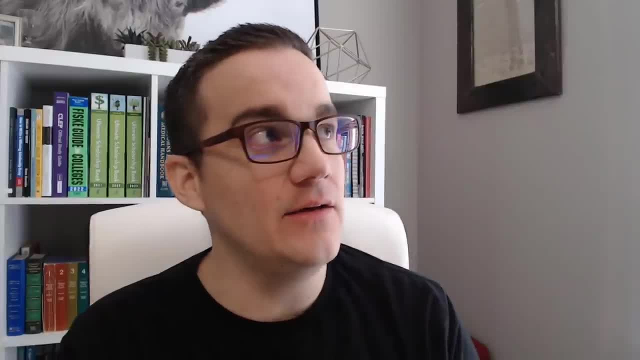 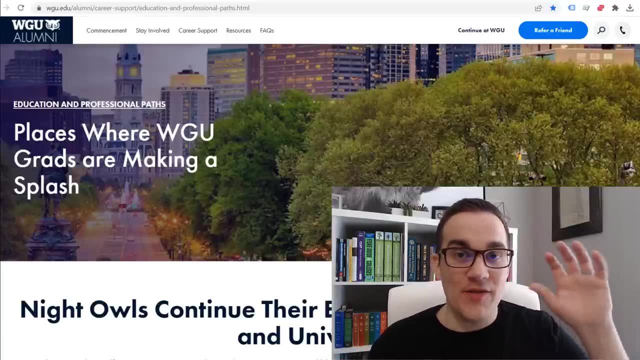 This is one of my personal favorite schools for accelerating. It's called Western Governors University. It's a hundred percent online. There's no brick and mortar campus, but they're regionally accredited and they're really really well respected. Okay, And here's. 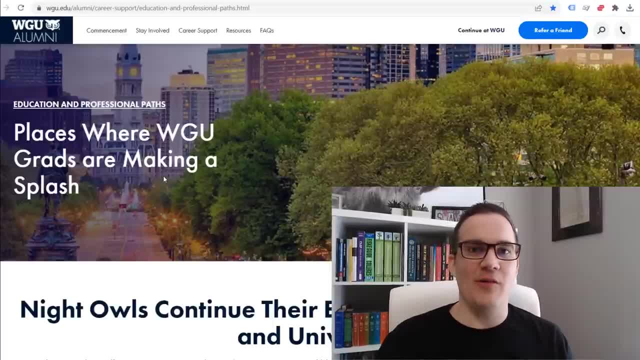 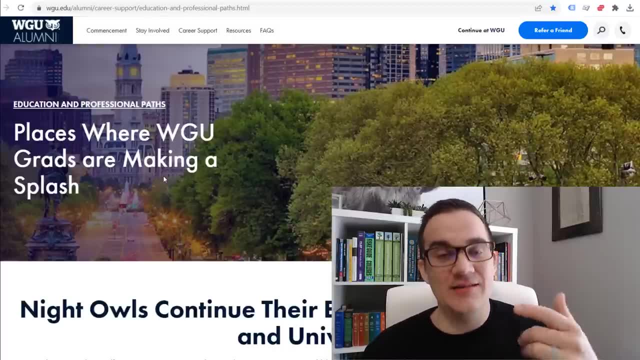 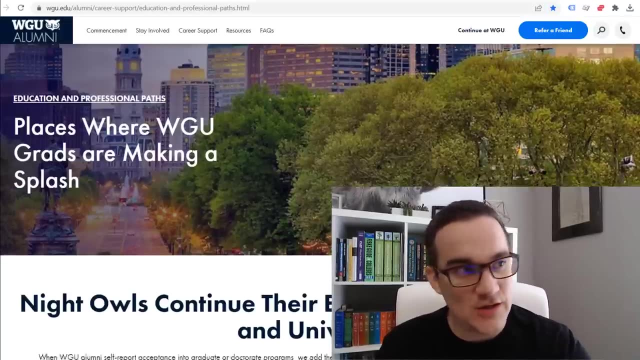 proof This is: I don't look for. Oh, if my friends haven't heard of the school, it's not a good school I look for. I look for job placement and placement into master's and graduate programs at prestigious schools. Now this is a page on Western Governors University's website. They have a list. These are: 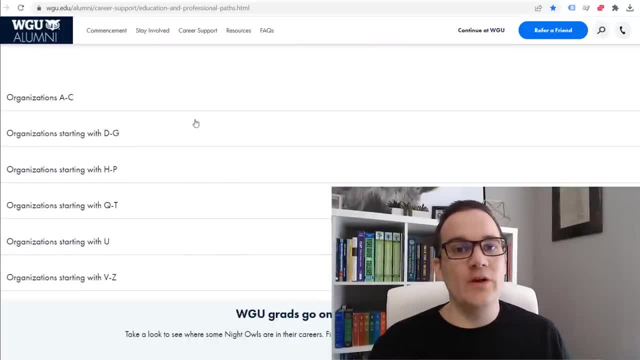 dropdowns. They have a list of really, really prestigious schools that have accepted Western Governors University graduates into their master's and doctoral programs. So what that means is, if you got a degree from this school, then you got into Harvard. They would put that onto this list- that Harvard accepts Western Governors. 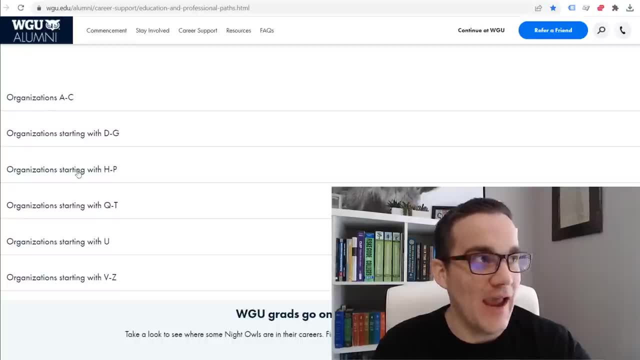 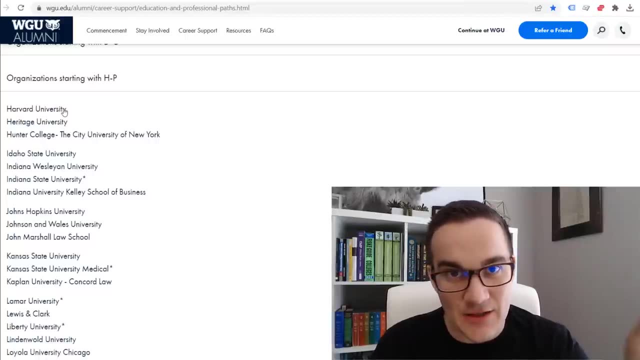 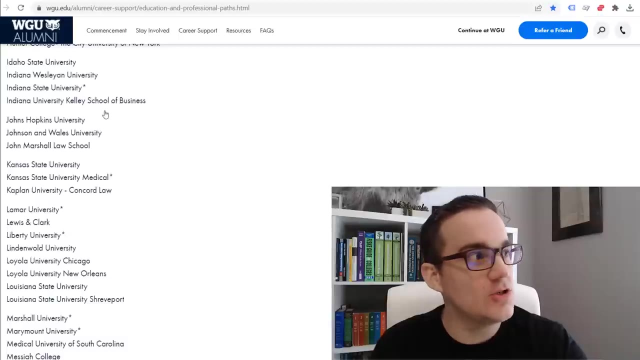 University graduates. So here's an example. We're going to just go to the H through P, because there's a lot of prestigious schools in this section. Harvard University has accepted WGU graduates into their master's programs. We go through here. Johns Hopkins University: super, super good school. 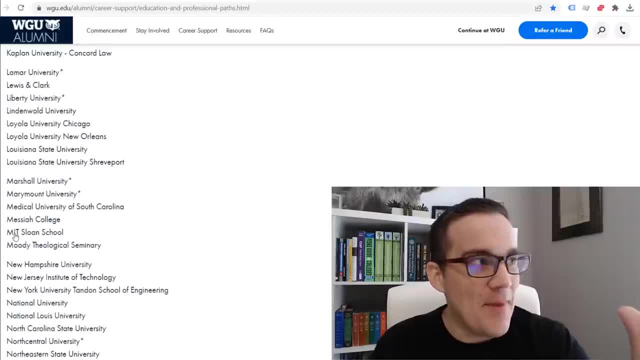 Loyola, super, super good school. MIT Sloan School. This is, this is MIT's business branch. They're they're business schools. So if you want, like a business degree or a management degree through MIT, that's what this MIT Sloan. 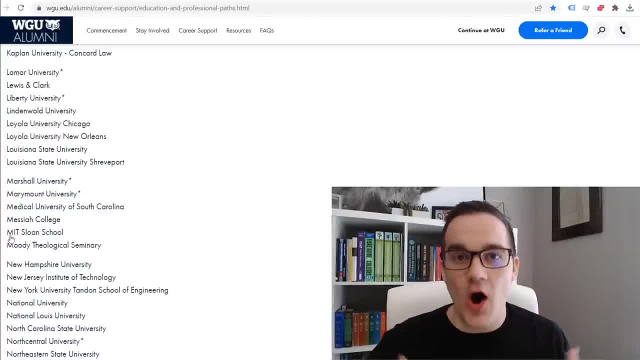 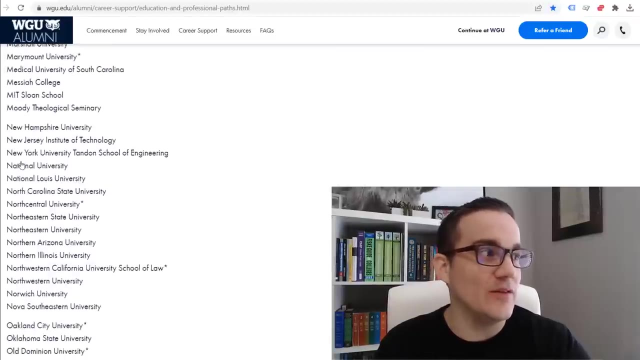 School is MIT, almost every year rated the number one most prestigious university in the United States. Sometimes the world has accepted WGU grads into their master's programs. Okay, If we keep scrolling through here, like just Penn State University, Purdue University, Princeton University, and there are 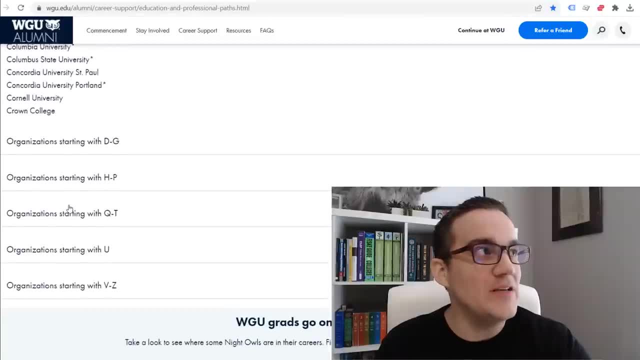 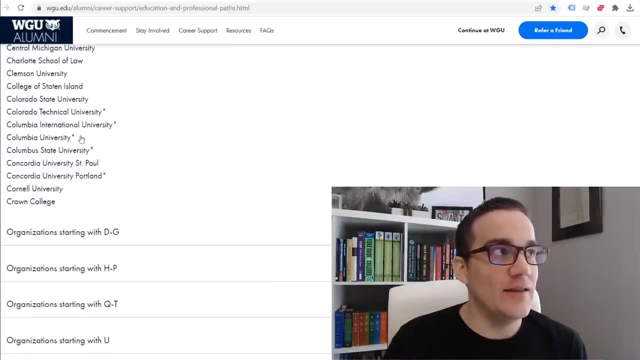 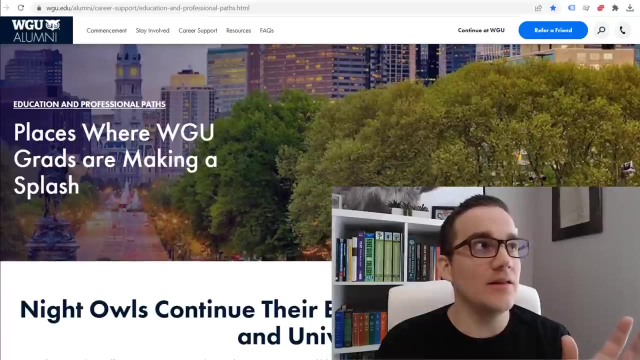 that's just H through P. Like there are so many schools in here- Cornell University, Ivy League, Columbia, ridiculous Columbia- they've accepted WGU grads into their doctoral programs. Like this is crazy. This- this shows you that. like it's a hundred percent online school. It's totally. 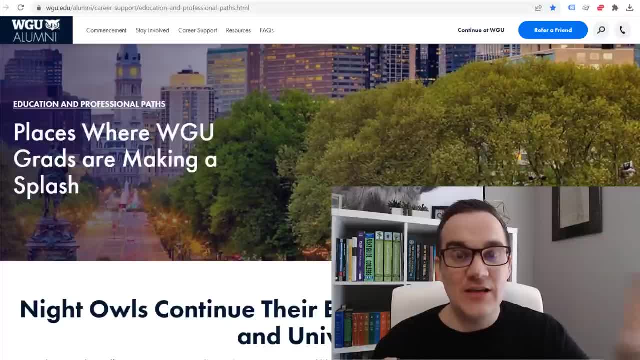 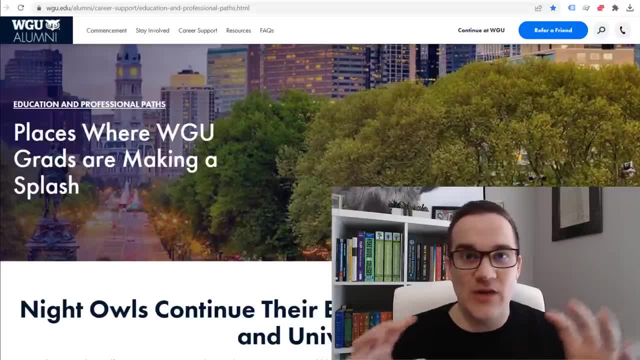 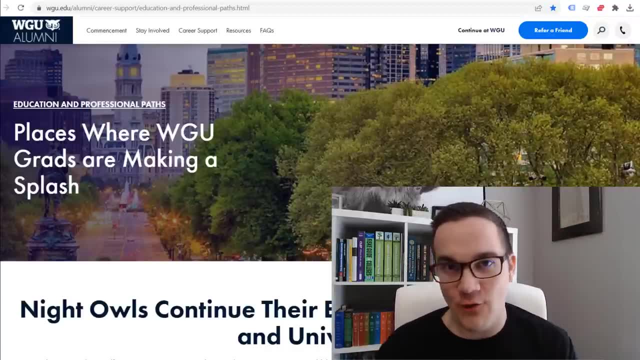 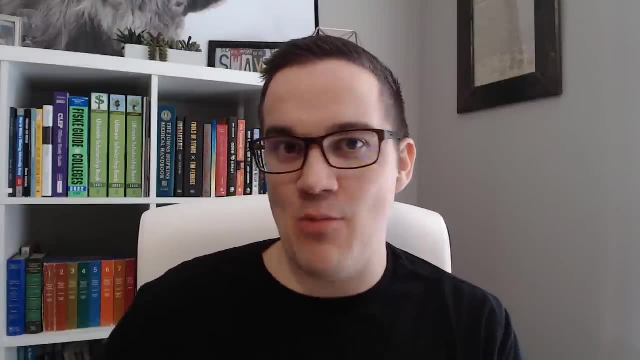 schools as equivalent to getting a bachelor's degree, like anywhere else. Okay, Their job placement's really good too, So these are good things to look for. when you're going through trying to find the right school, Stop looking at the name or if all your friends have heard of it. 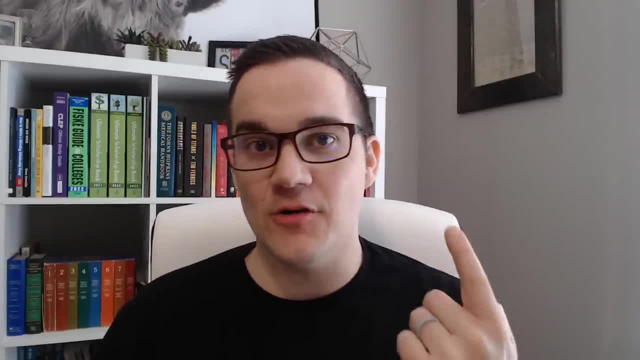 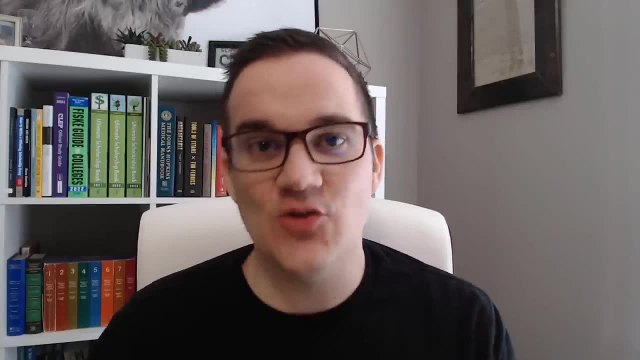 or if you love their sports teams and start looking for what is the fastest, most affordable degree that you can get, And if you're looking for a degree that you can get, then you're going to be looking for a degree that you can get. that's going to open all the right doors for me career. 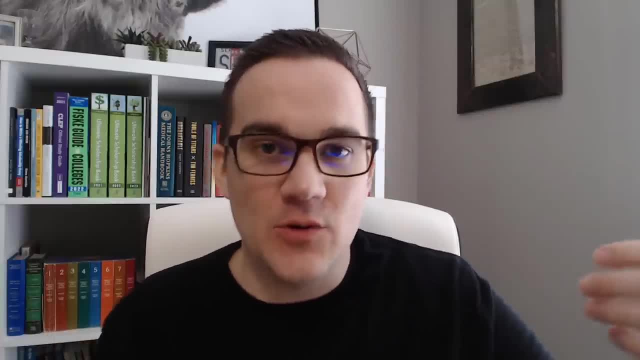 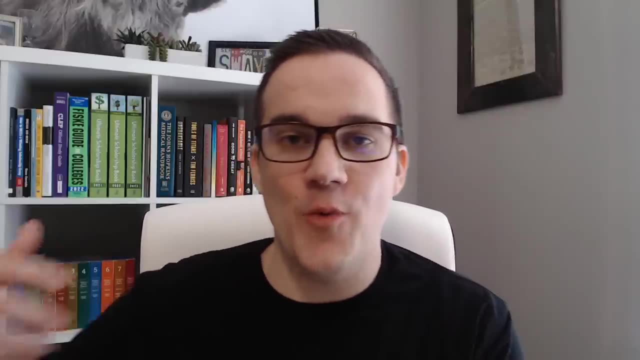 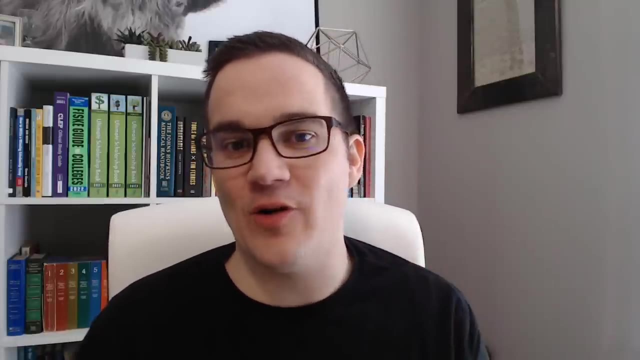 wise. That's what's important. Why do we go to college? So we can get better jobs, so we can have better careers. Okay, So look for schools that are going to open the right doors for the most affordable, fastest way possible. Okay, And the next thing I want to talk about, number four. 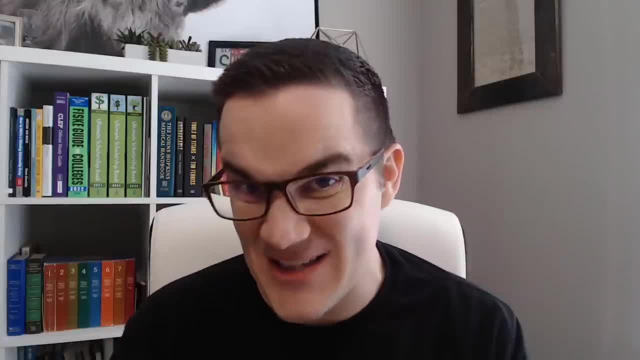 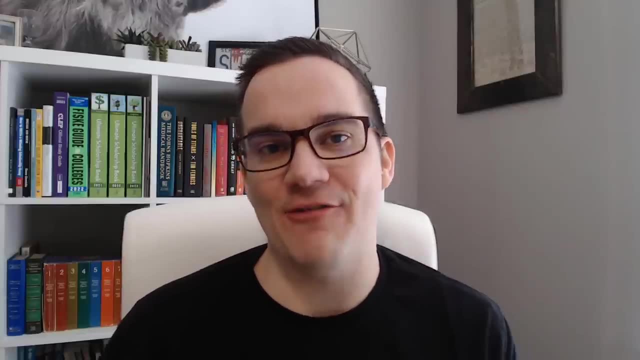 this is kind of a bonus. This will not help you graduate faster, but it will save you a lot of money on tuition, And that is if you're going to go to college you're going to have to go to. I like looking at schools that offer flat rate tuition instead of schools that charge per class. 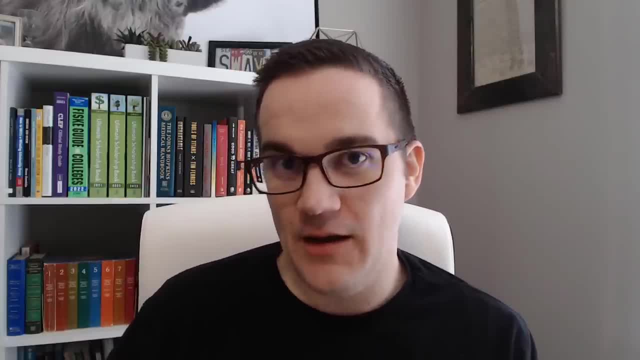 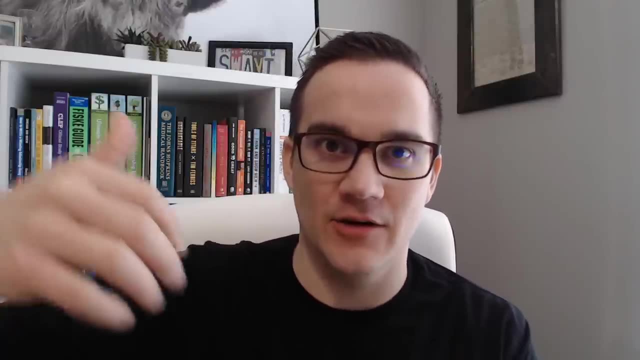 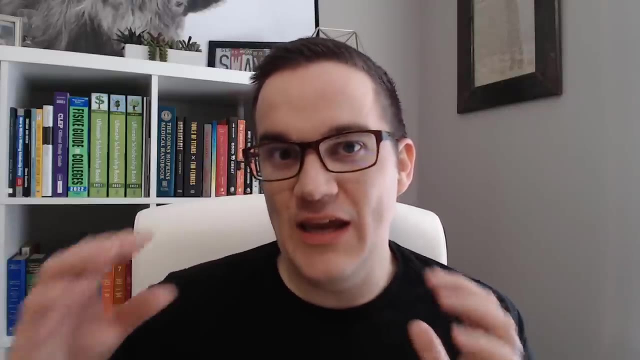 or per credit. So what most schools do, it's like 120 credits to get a bachelor's degree, depending on the credit structure. Some schools will say like 180, but their credits are like smaller 120 credits. for a bachelor's degree, We charge $500 per credit. Well, if that's the model of how they charge you as a student, then you're going to have to go to college. If you get earn all those credits in six months, you still have to pay $500 for per credit for 120 credits, Like you're still paying for a four-year degree, even if you get it done in six months. 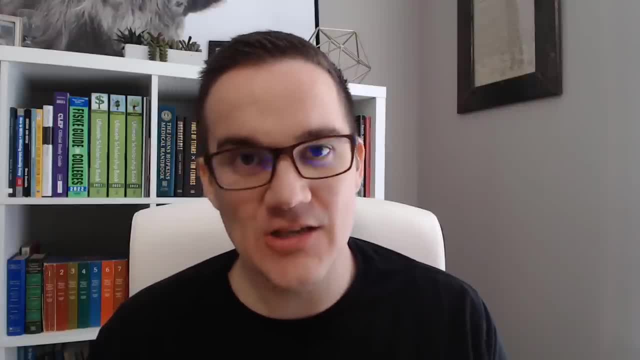 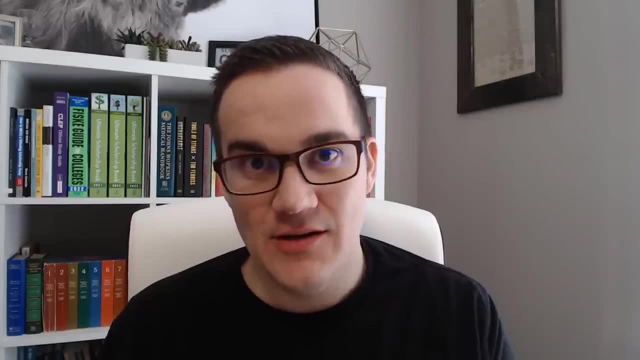 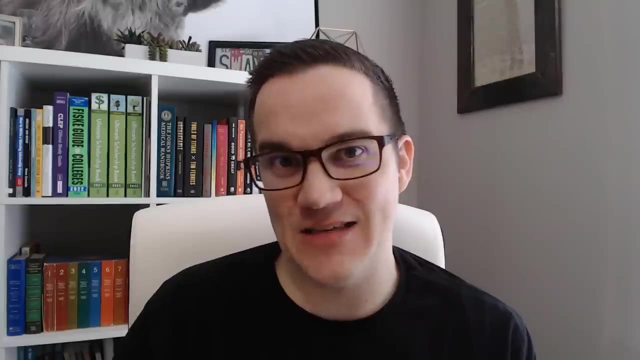 schools that offer flat rate tuition. essentially how it works: You pay for a semester and then you finish as many classes as you, as you want, in that semester, And the price is exactly the same. So whether you finish four classes or 40 classes, it's the same price for that semester. 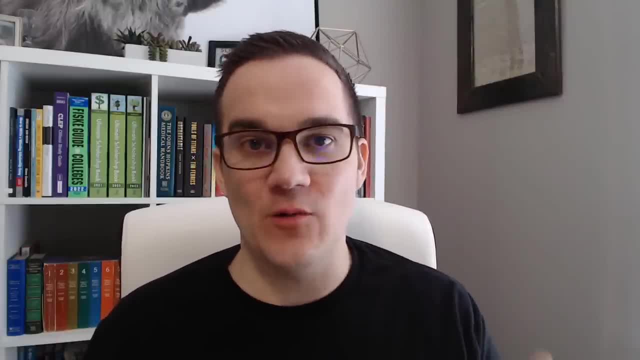 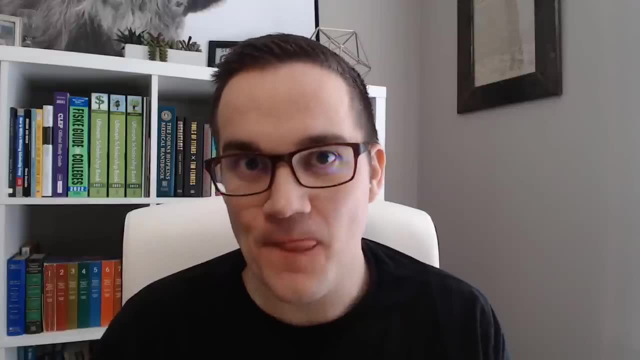 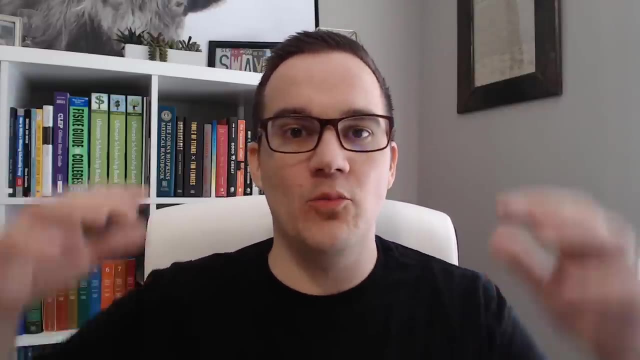 Well, when you do that, you get to the point where, like, if you graduate, get a degree in six months, you're paying like three to four grand for your entire degree. If you graduate in a year, you're talking seven to $8,000 for an entire bachelor's degree. Well, when you bring 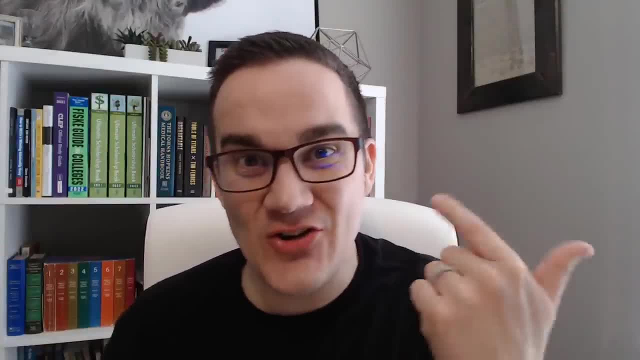 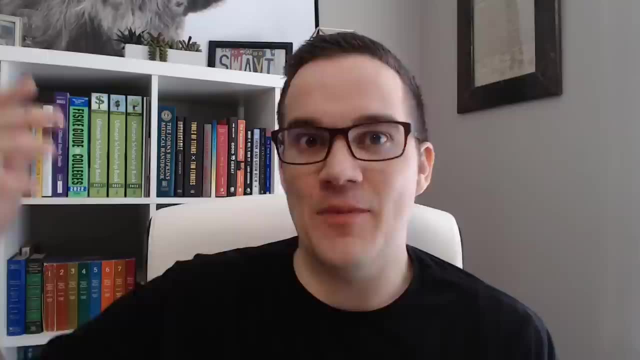 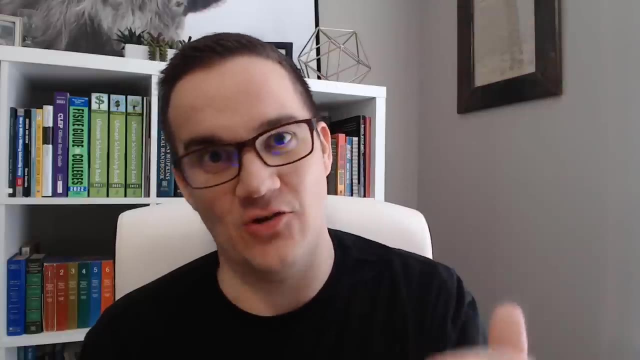 the price down that low. scholarships and grants- like. coming up with five grand in scholarships and grants is really not very difficult. Coming up with a hundred thousand dollars in scholarship grants and grants is really really hard. So if you can bring the price down, 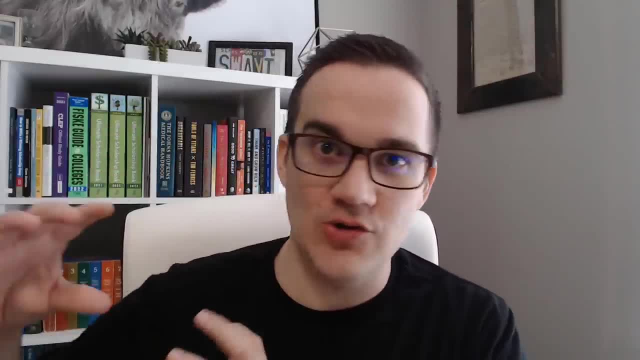 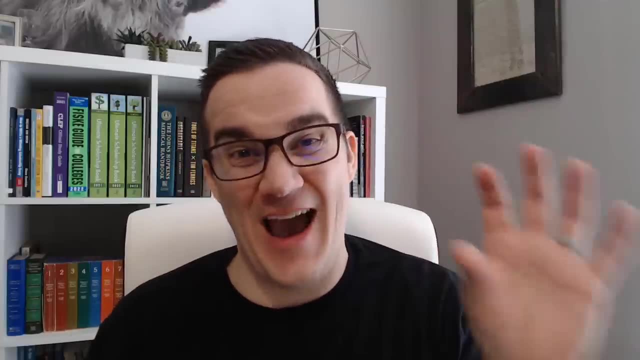 graduate in less than a year. you can usually make scholarships and grants, pay for a hundred percent of your tuition and you're not out of pocket at all. So this is my process for how to find schools that will allow you to graduate in like as little as three to six months with a 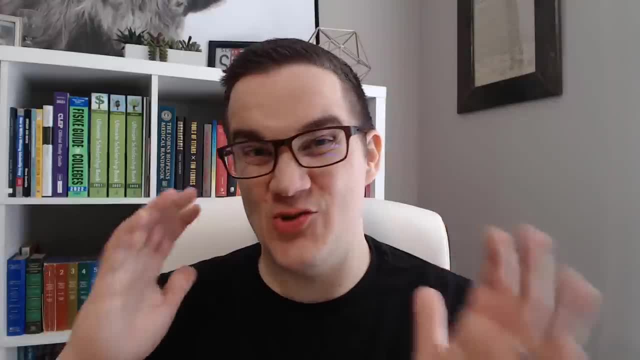 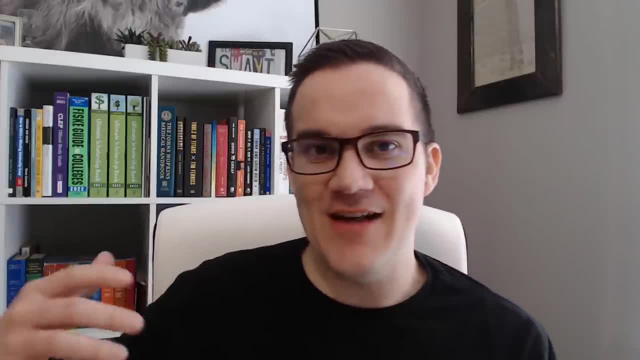 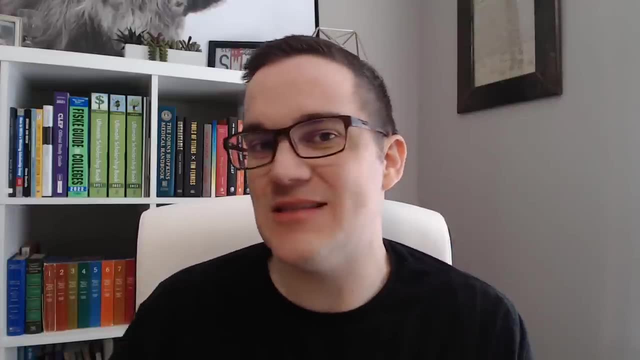 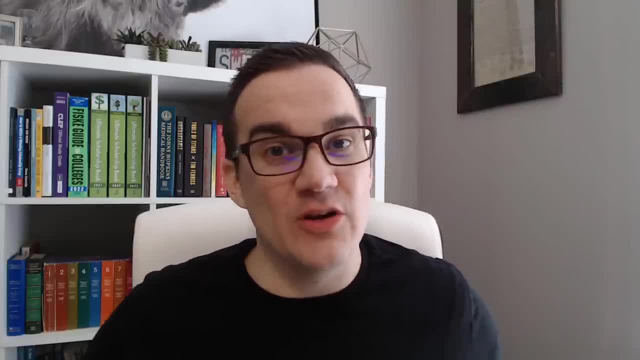 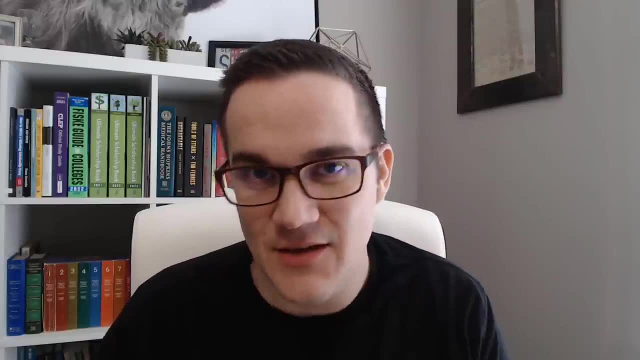 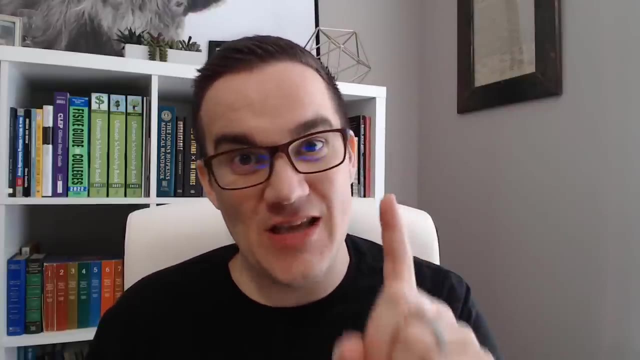 six to 12 months is the goal. You can do this really really quickly, qualify for your dream job faster and not be in a huge hole of debt. So it's a much faster process. I hope this video has added value to your day. Choosing the right school is just step one of the process. Like once. 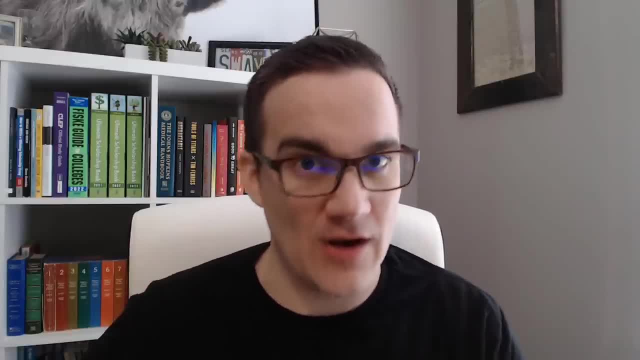 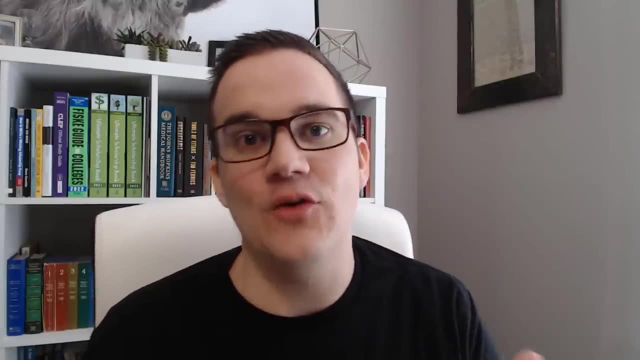 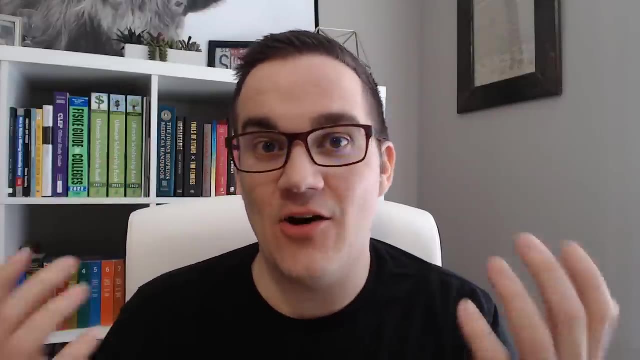 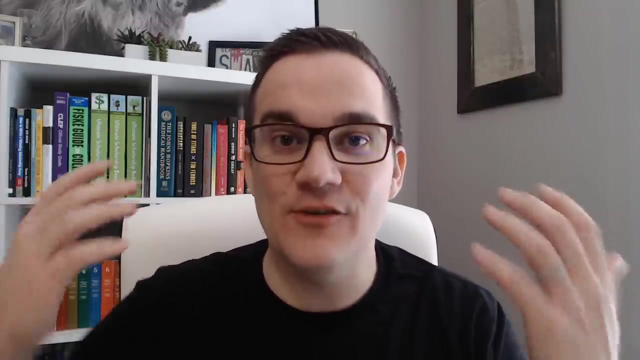 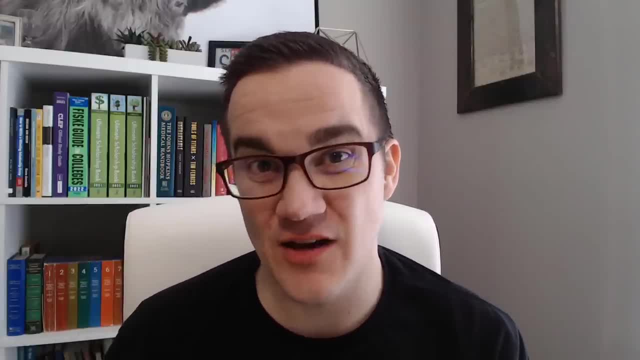 about how to get college degrees faster and how to save a fortune on tuition. I hope you have a wonderful day and I will talk to you in the next video.